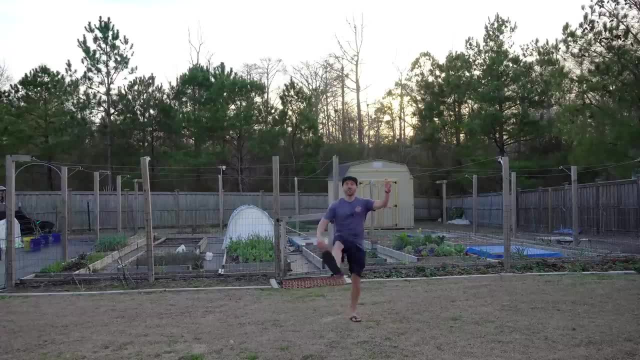 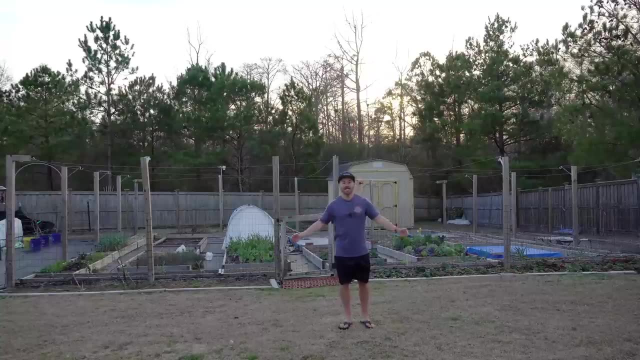 I moved here was for the warmer weather, more sunshine and to wear flip-flops all year long, no matter what the weather or the season. So I purchased this property in 2018, and when I purchased this property, it was nothing but a clear-cut sandy lot. And, much to my chagrin, it was infested with biting ants and fire ants. Anytime I'd go outside in my flip-flops, I would get bites on my ankles and in between my toes. My dream of wearing flip-flops. 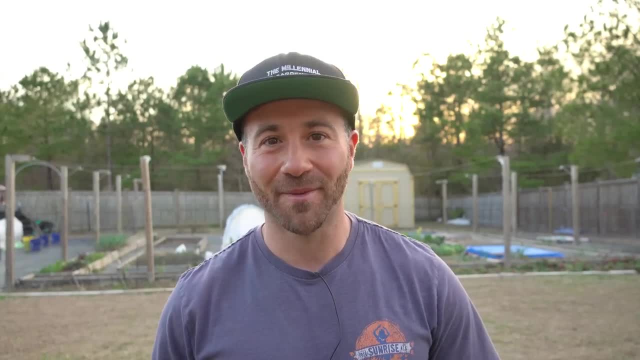 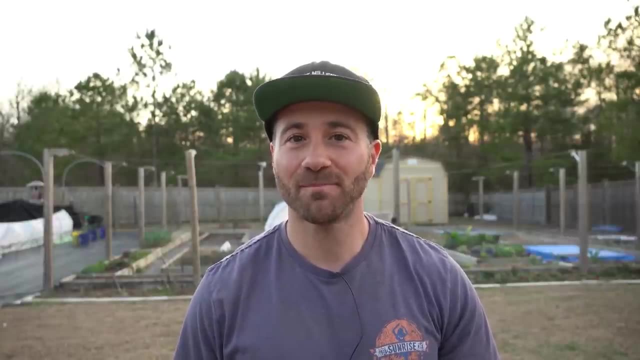 all year round was shattered and I knew I had to do something about that. Simply targeting and destroying the ant colonies was not working. Every single time I'd destroy one, two or three would just pop up right next to it. I had to figure out why they were coming and solve the problem. 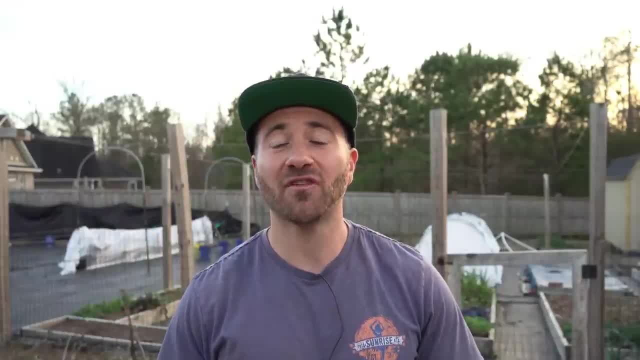 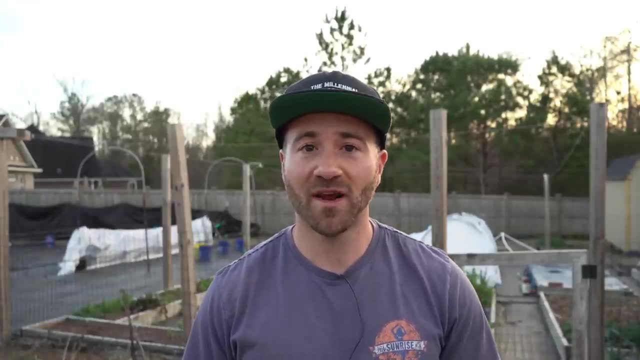 I'm an engineer by trade, so I put on my engineering hat and what I figured out was the problem was my soil itself. Here, where I live, I have very firm, sandy, well-draining soil. That is exactly what ants want to build their colonies in. 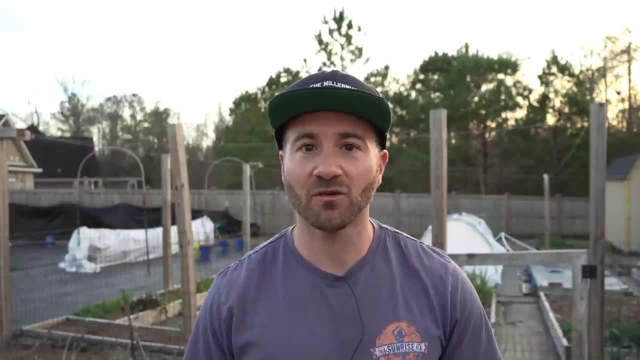 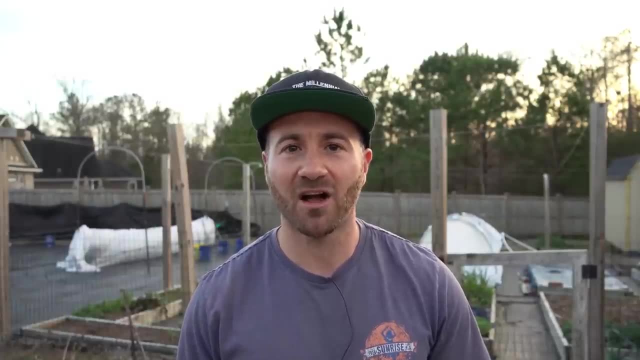 because it holds shape. They can dig those intricate networks of tunnels and not have them collapse. So it didn't matter how often I would try and destroy and police my yard for these ant colonies, because they would just keep coming because the soil that made 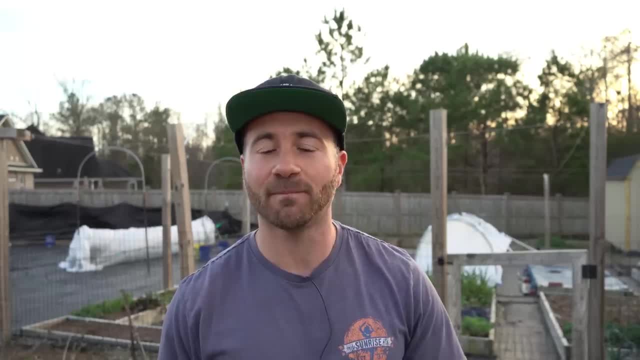 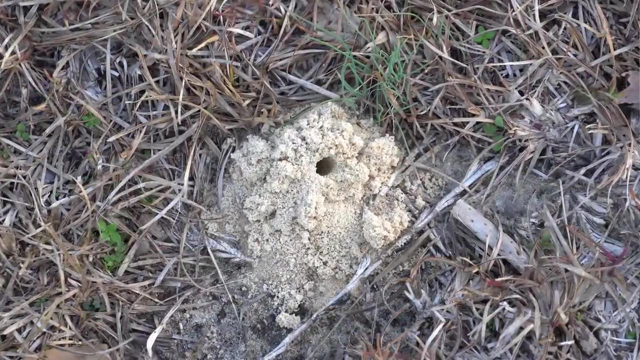 up my yard was a gold mine. It was exactly what they wanted to build their nest in. If you go searching your yard for ant hills, you will find the mounds around the ant hills always look like perfect sugar sand, like you purchased a commercial bag of play sand from a big-box store. 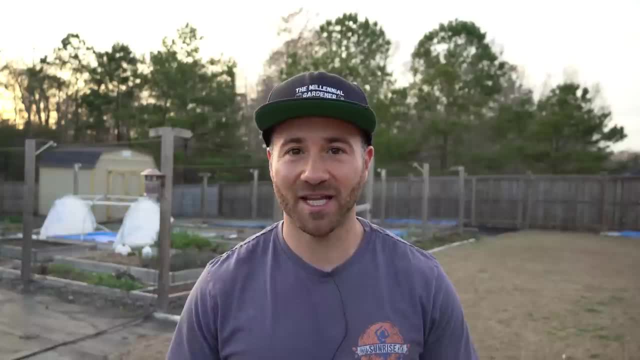 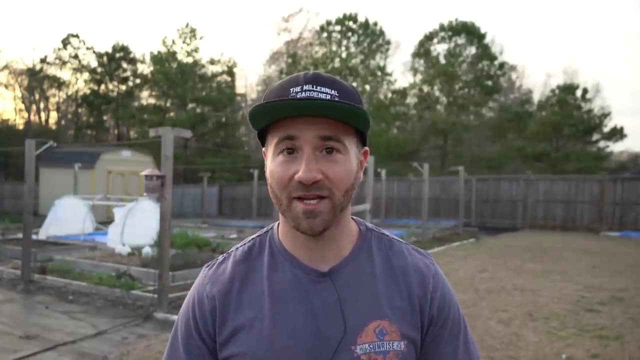 that you would fill a child's sandbox with. If this soil type is present in your yard, ants are going to flock to it because it holds the shape of their colonies perfectly. So you need to deal with that reality, and I have a three-step process that will help you accomplish. 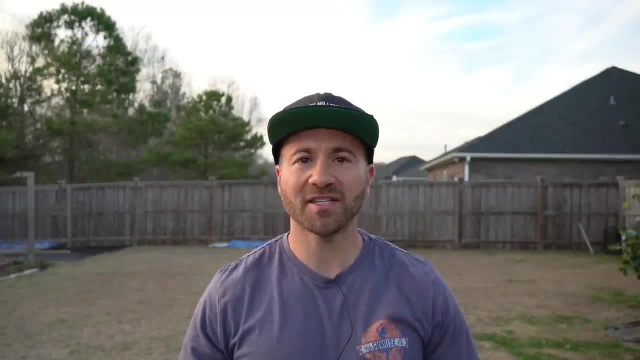 this. The first step will be a defensive strategy that will try and dissuade ants from coming onto your property. The second step will be a defensive strategy that will try and dissuade ants from coming onto your property. The second step will be a defensive strategy that will try and dissuade. 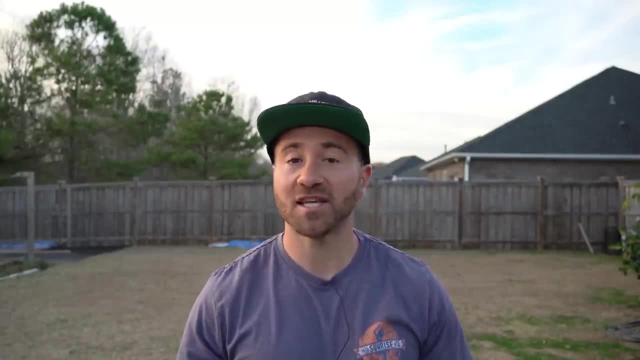 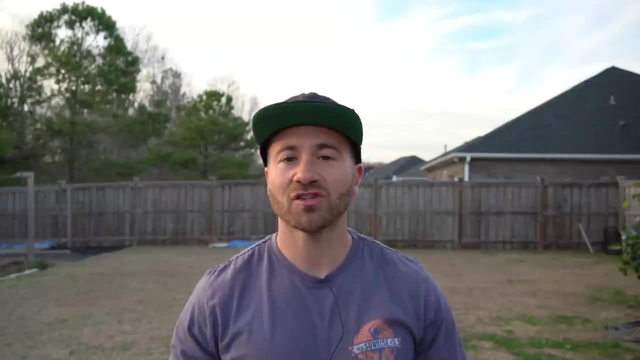 your property. The second step will be an offensive strategy to help deal with the ants that do slip through your defenses, and the third step will be a long-term, transformational strategy to change your yard so ants will no longer ever want to take up residency in your 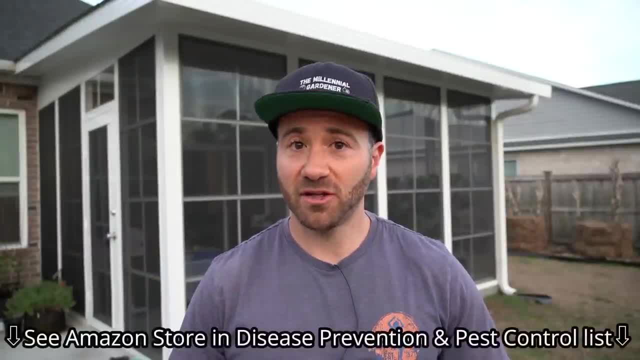 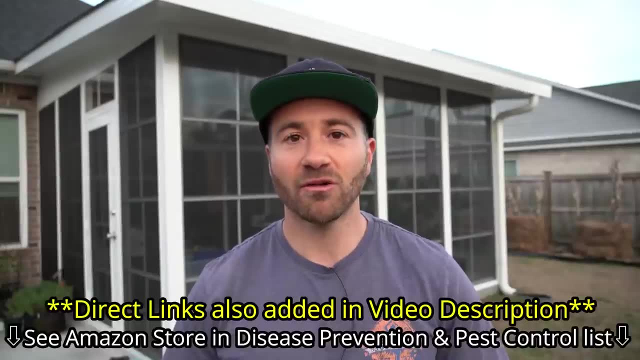 yard and garden. again. For your convenience, I'll make sure to link the products that I use in this video down in my Amazon storefront in the video description Underneath the list disease management and pest control. I'll also put a couple of direct links in the video. 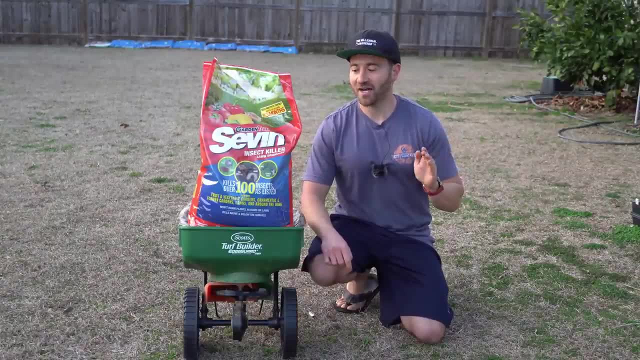 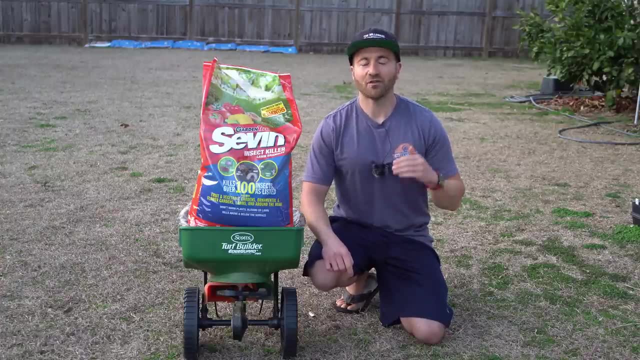 description as well. The first step is going to be your defensive strategy. If you're a gardener, you're going to want to have a defensive strategy, and that is going to be to spread insect-killing lawn granules around your lawn with a spreader, And the reason why you're doing this. 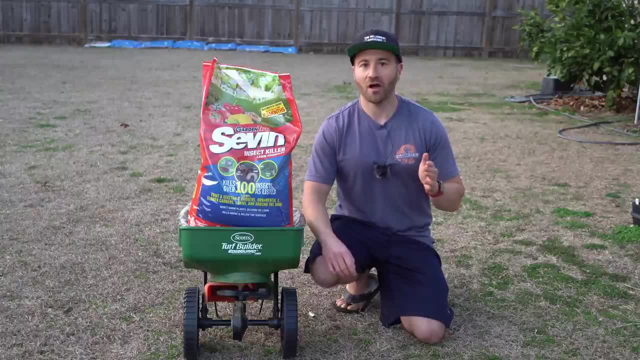 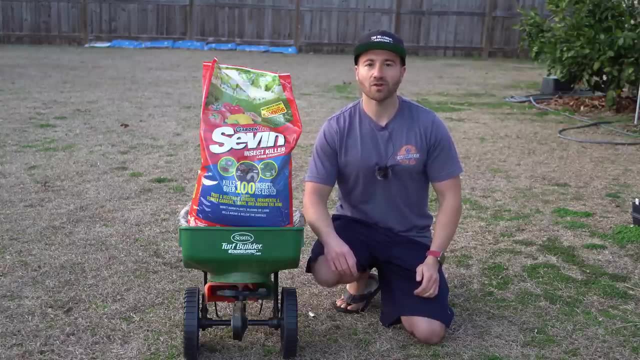 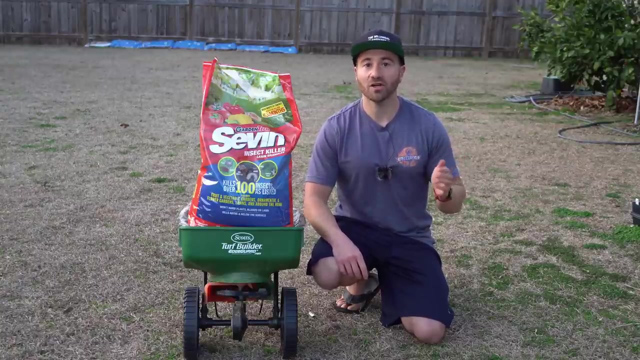 is you want to create a barrier of sorts around your yard. These granules are made out of synthetic pyrethroids, which are contact killers for almost all insects, So when you spread them around your lawn for any scout ants that are looking around trying to locate a good location to set up a new, 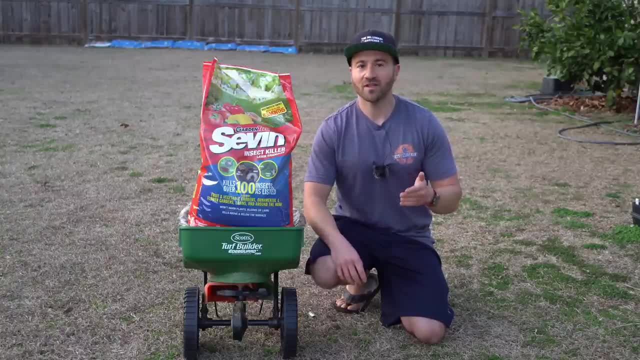 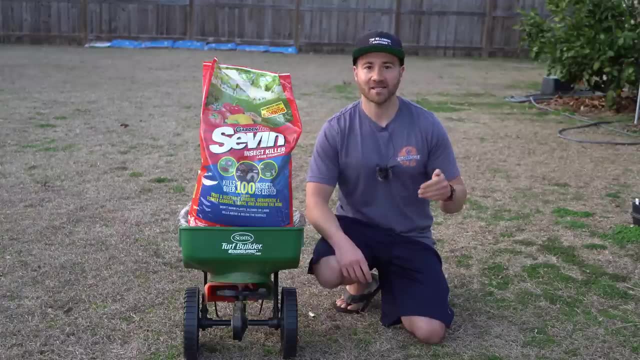 colony, they will, over the course of a year, they will be able to spread insect-killing lawn granules around your lawn, And then they will die, So they won't be able to go back to wherever the main nest is and alert all their friends to build a new home on your property. Now, when it comes to application, 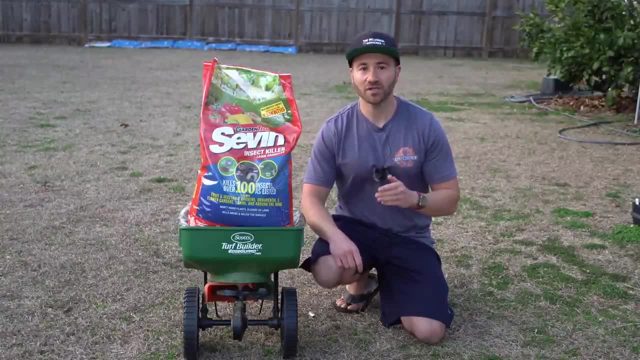 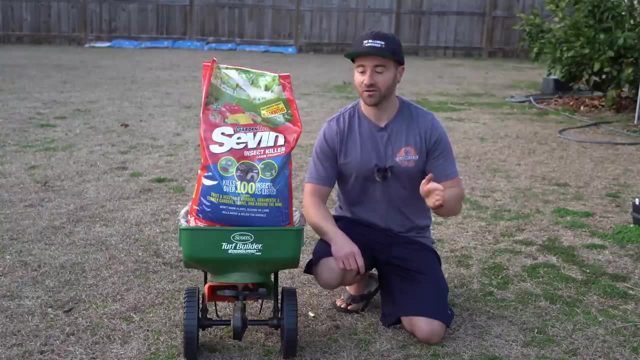 schedule. everybody needs to make their first application in late winter or early spring, right around the time that insects are going to start coming to life again, because you want to defend your yard and garden. These last for up to about three months, So for most of us, we will all. 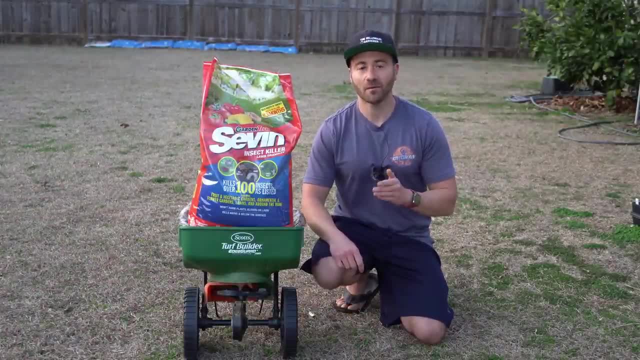 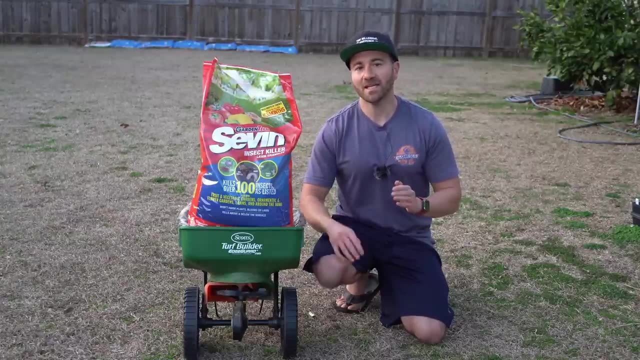 have to make an application again right in the beginning of summer, which will be three months later. Then, for those of us with very long growing seasons that live in the deep south, we may need to make a third application in the fall again For those of you with shorter seasons that get frost. 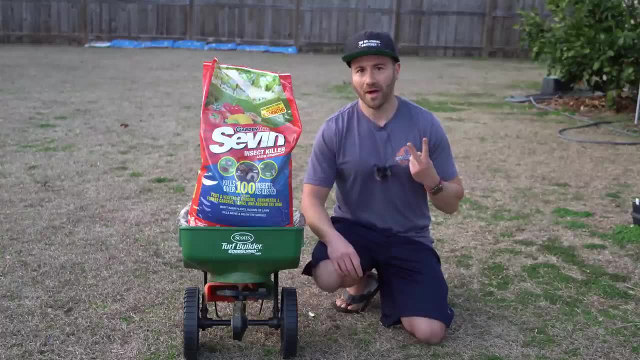 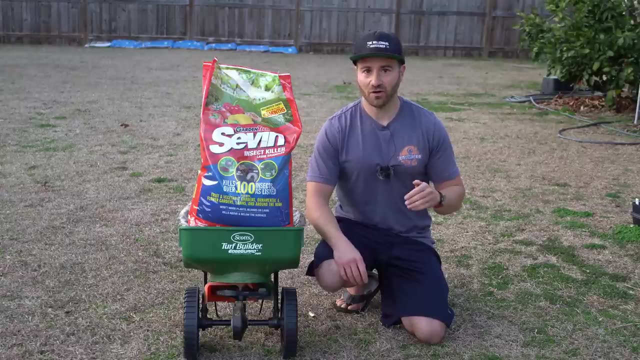 in September and October. you may only have to go with two applications a year And when you spread these granules all around your lawn, that is going to be your defense for your yard. That is going to keep most of the pests away, especially if you're going to have to make a third application in the 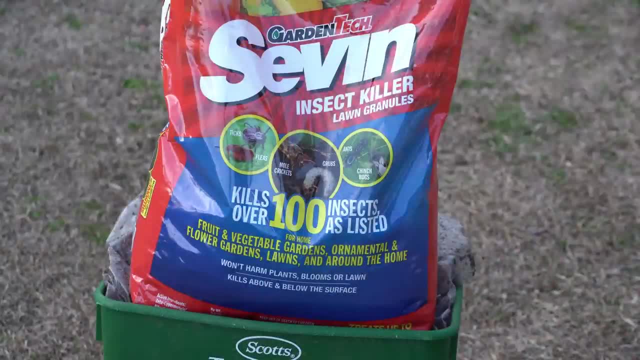 But before you go and use these synthesized pyrethroid granules, you have to understand a few things. You can only apply these to your lawn. You cannot apply these to your garden, despite what the bags say. If you put these in your garden, you can have detrimental long-term effects. Synthetic. 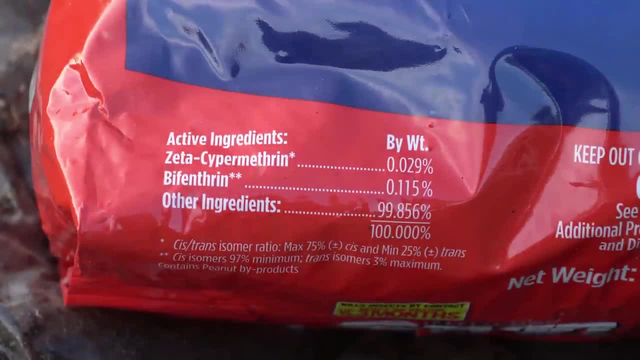 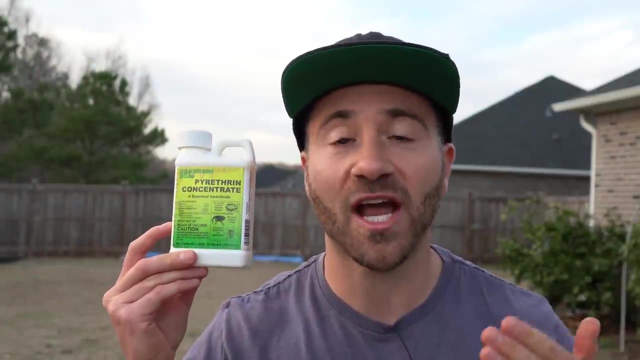 pyrethroid granules are created in labs to mimic the toxic effects of pyrethrin. Pyrethrin is a natural extract made from the chrysanthemum flower And if you follow my channel you know I use natural pyrethrin in my garden all the time for insect control. in the dead of summer, when my 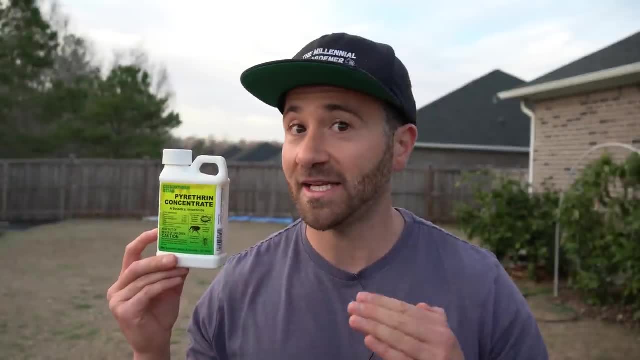 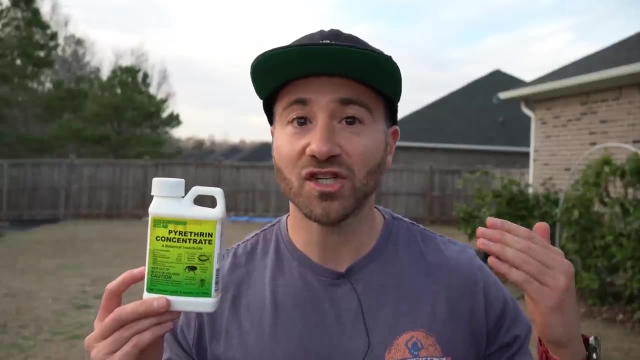 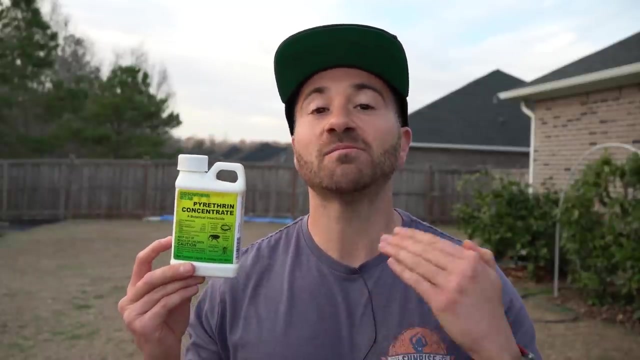 insect pressure here is off the charts. Natural pyrethrin is a natural product And as a result it's very prone to oxidation. So sunshine and fresh air- oxygen- will oxidize it and decay it rapidly. So when I spray my garden after sunset it is mostly burned off by the morning, and any 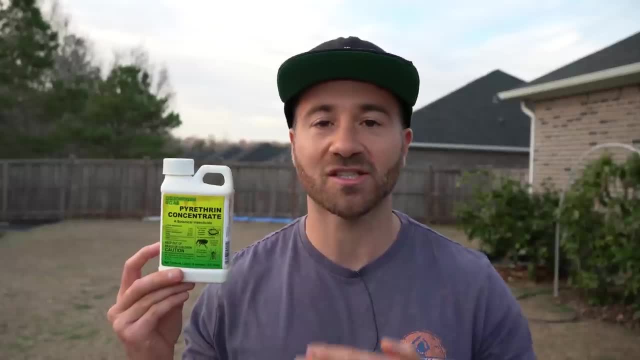 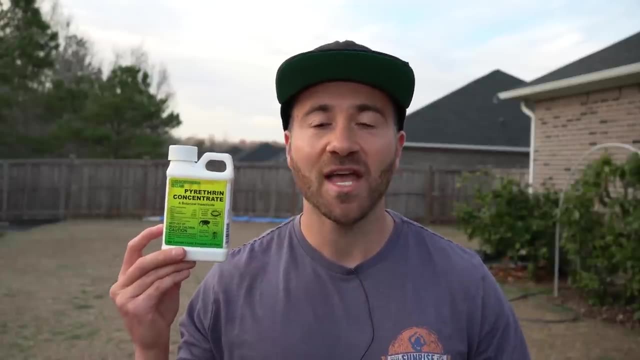 poison that is potent will burn off as soon as the sun rises, So it's completely safe to eat your vegetable garden the very next day after you spray with pyrethrin. because the half-life is so rapid, It decays very quickly. Synthetic pyrethroids, on the other hand, 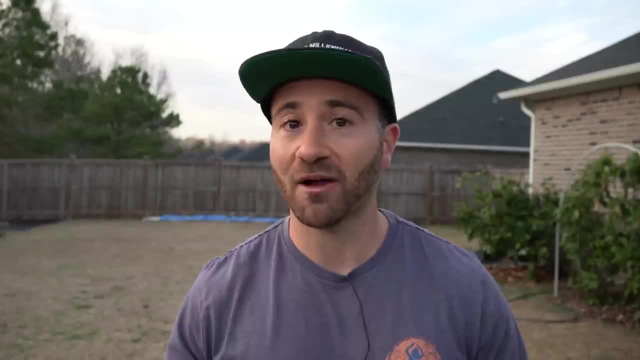 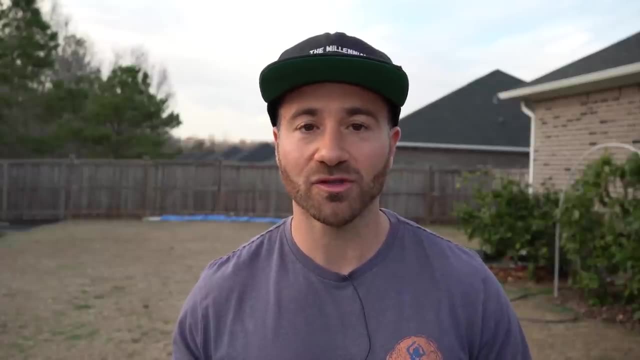 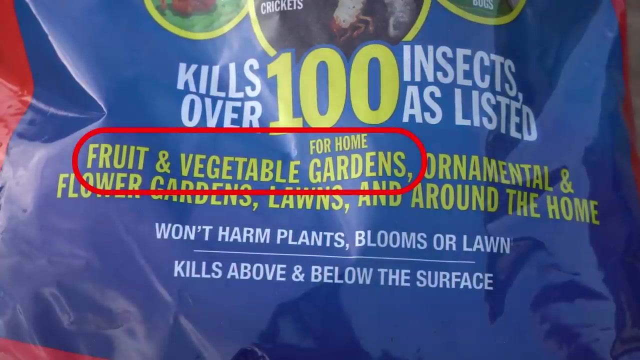 are made in laboratories to have the same effects as pyrethrin, but to last for months and months. They're made to resist oxidation, So when you place those granules on your lawn, the toxic effects will persist for months. Now, while it does say on the bag that it's safe to use in fruit and 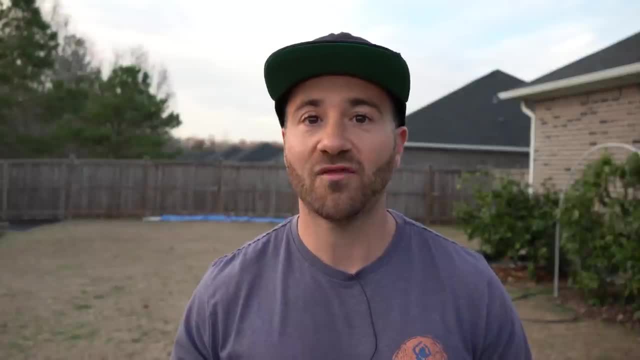 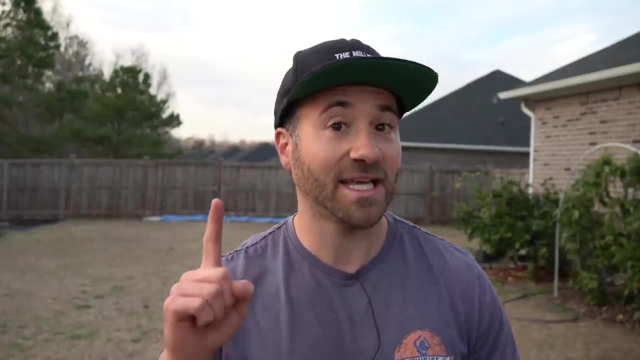 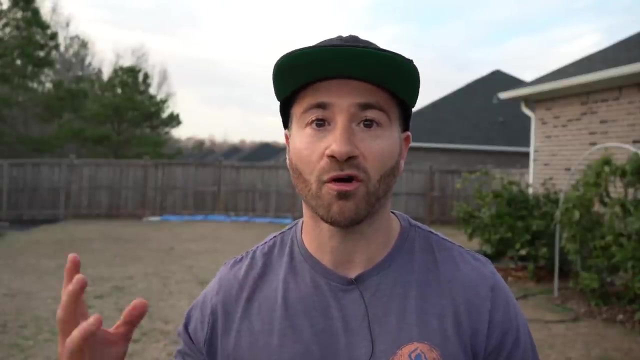 vegetable gardens. that's only because pyrethroids and pyrethrin is very low toxicity to human beings, But it is extremely toxic to all insects and actually cats as well. So, while it's safe to go out in your garden and spray after sunset a natural pyrethrin product, because it'll burn off, 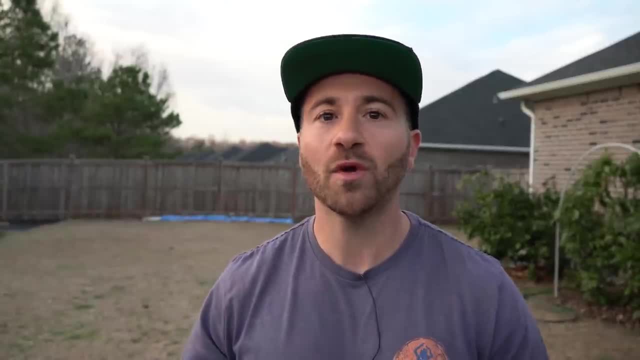 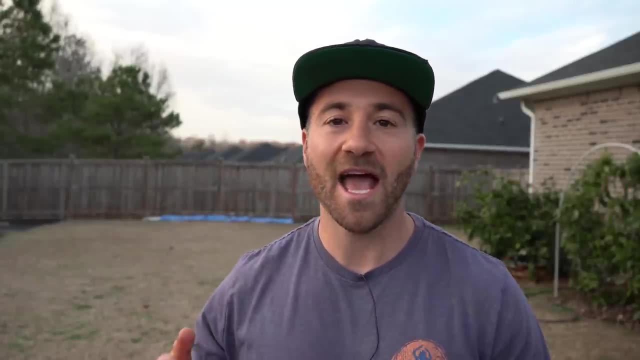 by the morning, by the time all the bees and the good insects come back. when you spread those granules in your garden, they will make your soil toxic to insects for months. So you'll be killing and all your good beneficial bugs in your soil that are composting things for you. So never put. 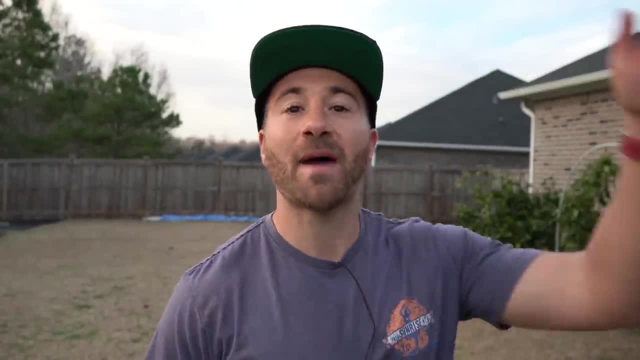 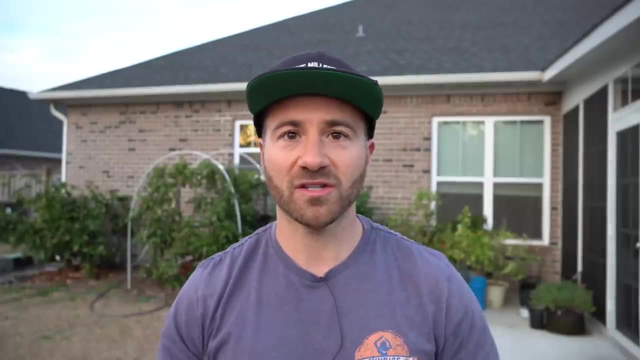 that stuff in your garden, Only put it in your lawn as a barrier around your property. Now you may be asking: well, if I put it down on my lawn, aren't I killing a whole bunch of earthworms and other good bugs too? And to that I'm going to say: possibly there is some risk to that. 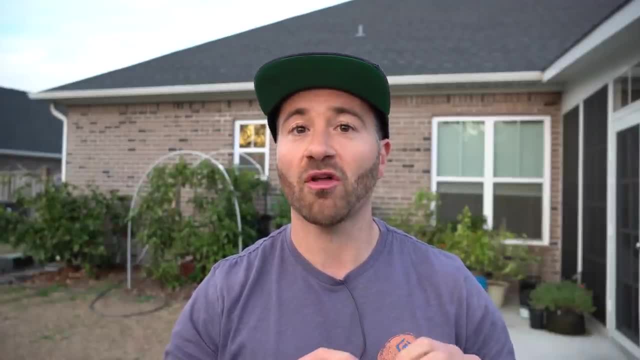 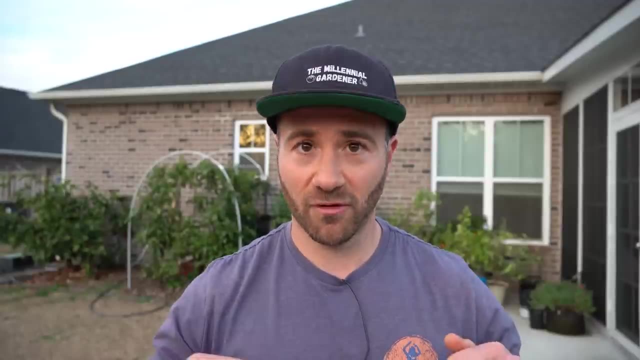 Generally speaking, it is going to kill the insects that are crawling along the surface of your lawn and that are only a few inches deep. Earthworms usually are several inches deep into the soil and the poison may not penetrate that far. So in my 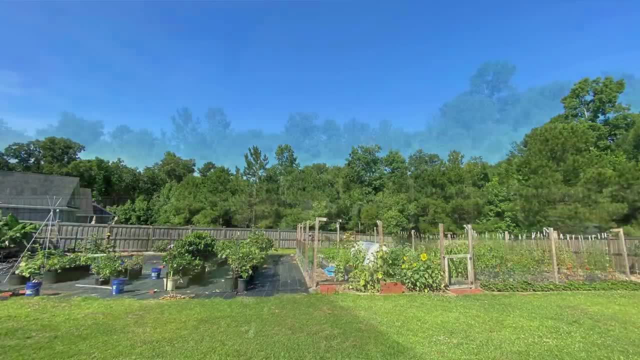 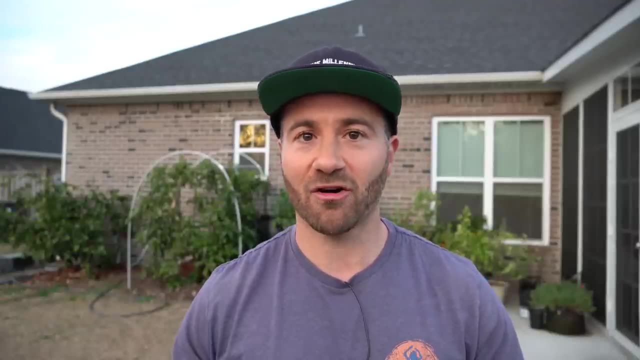 experience. my garden is in the middle of my yard and the earthworms make it down probably pretty deep across my lawn and into my garden. no problem, My entire garden area is just teeming with earthworms, So using those granules on your lawn only seems to be relatively low risk. It. 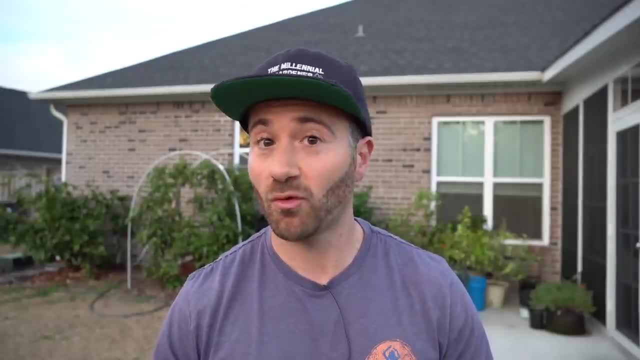 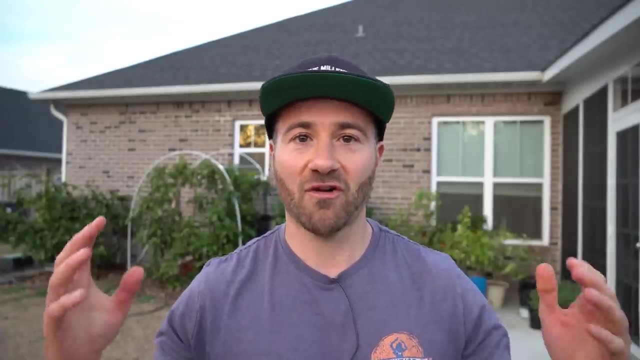 probably will kill some, because nothing is ever 0% or 100%. But if you have this big problem with ants and other pests, you may not have a choice. So you really have to weigh your options here. There is no perfect answer here, but I think this is the best method for people. 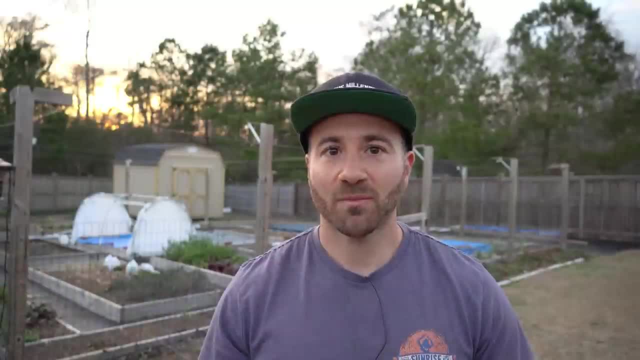 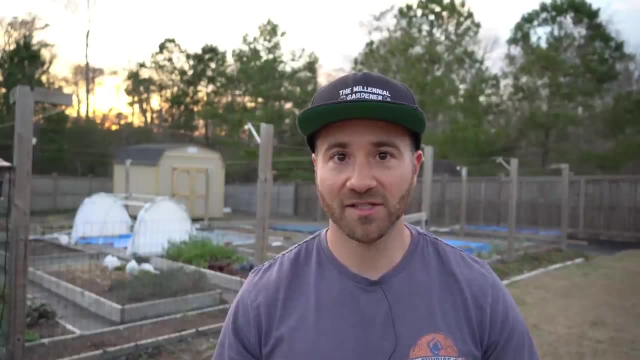 with really bad problems with ants and other bugs. Now, as I previously mentioned, no defensive strategy is 100%. Eventually, some ants will find your yard, They will make it through your defenses and they will take up residency. So what you want to do is have an. 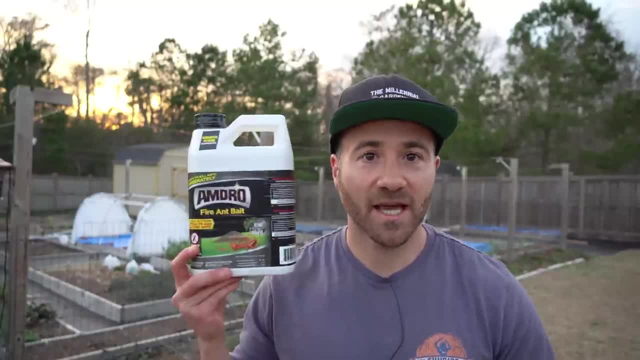 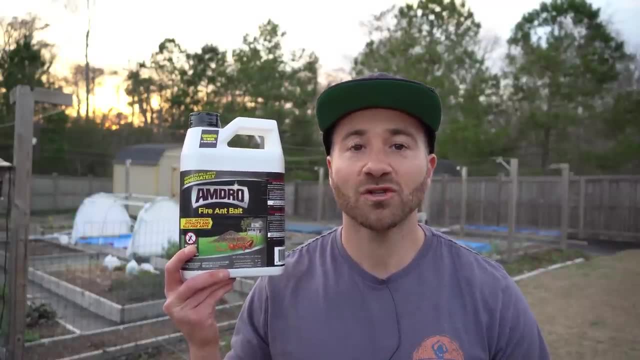 offensive strategy. And that leads me to my second tip: Get yourself an ant bait product like this. Ant bait products are fantastic. They are specifically designed to destroy colonies, And what they are is: they are a poison that is very attractive to the ants that they think is. 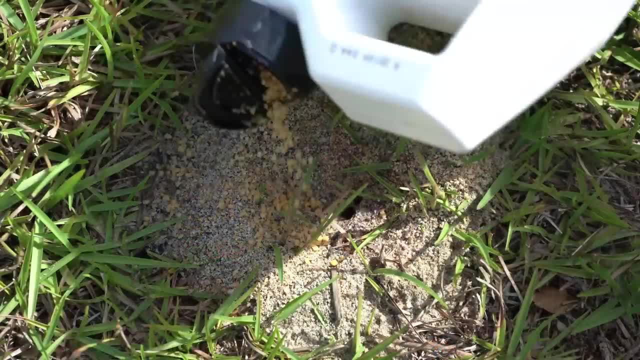 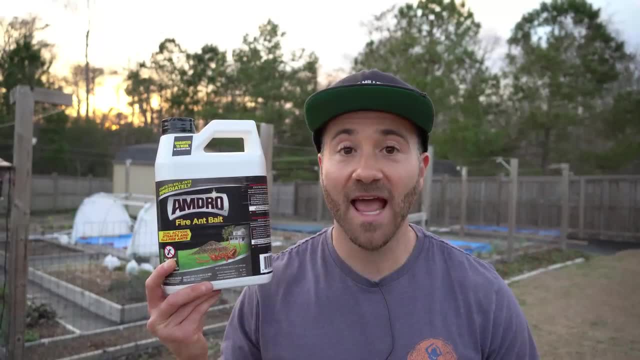 food. So all you have to do is put one teaspoon of this product right outside of their ant hill, a few inches away, and the ants will come out and greedily take it back to all of the other ants and the queen in their colonies And they will all feed on it, And in a matter of 24 hours. 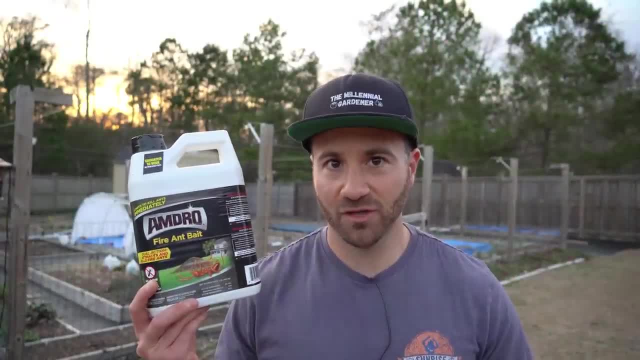 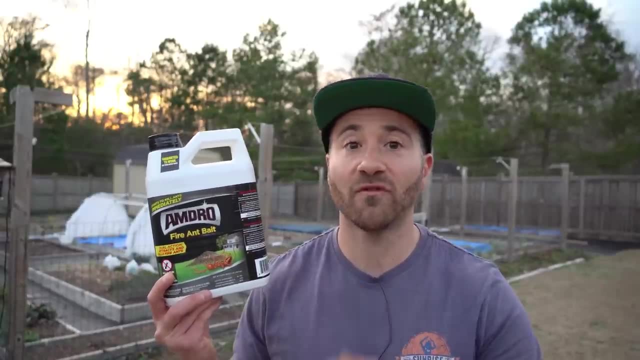 it will kill the entire colony. Once you spread those lawn granules and you get an overall handle on the insect population in your yard, you then target any colonies that do pop up and they kill them very quickly. Now I will say there are natural alternatives, that 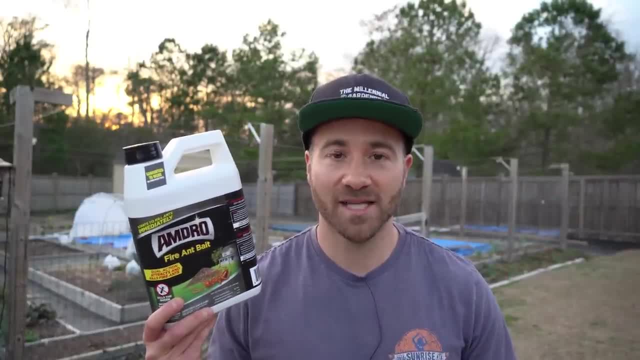 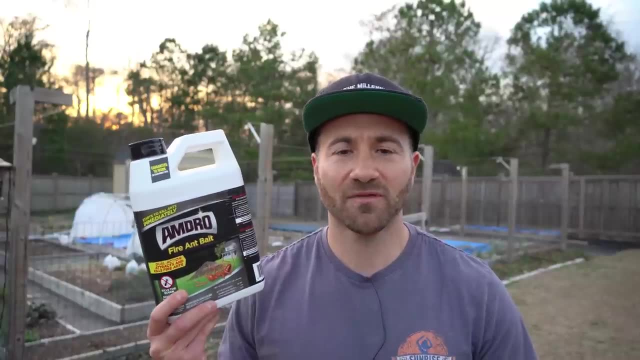 you can use. instead of using this product, You can make your own mixes out of borax. However, I will say that these products work a whole lot better and they're a lot more convenient. This jug right here was only a couple of dollars, and there's still plenty left. And this is my third. 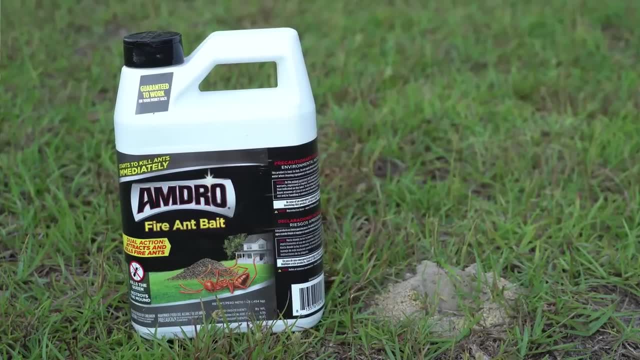 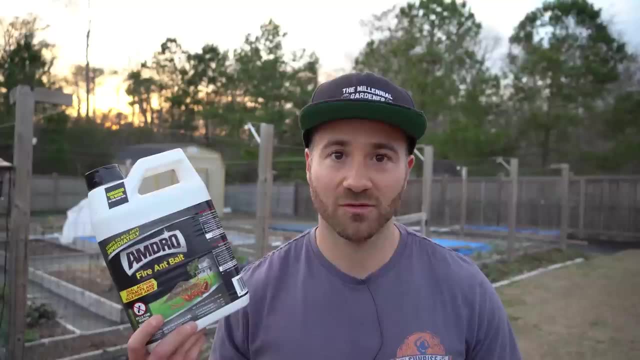 season that I'm using it. So for a $10 to $15 investment, you can go for many years with a very natural product like this. If you want to go the natural route, you can look up recipes for making your own borax solution as well. So what I do is, once a week I take a walk around my entire yard. 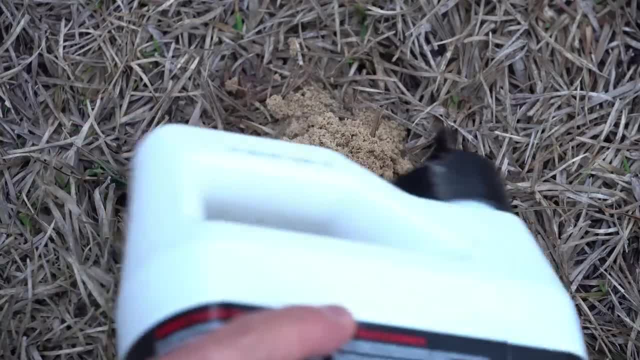 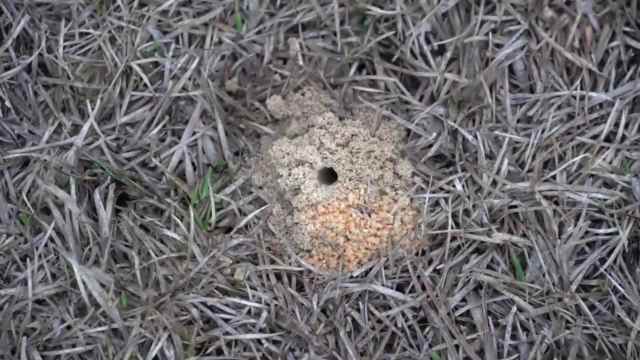 and I search for any ant hills that may have slipped through the cracks And I put about one teaspoon of the granules next to the ant hill, And the best time to do this is first thing in the morning when the sun rises, because ants are most active in the morning. Up until this point every 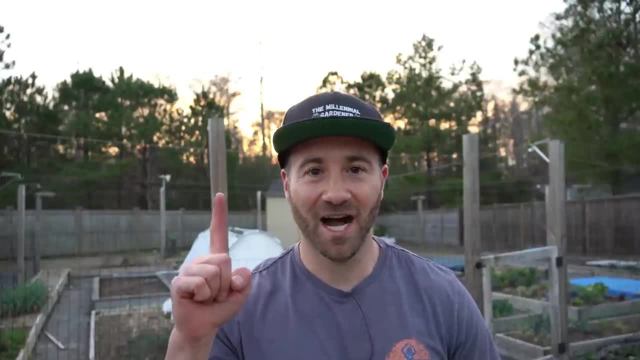 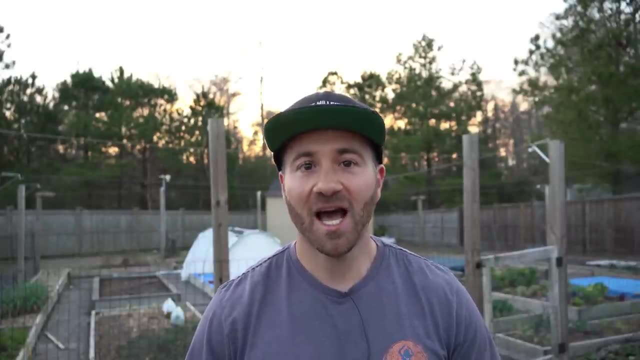 single ant hill that I've shown you in this video so far all have one thing in common: They are all from my front yard. I can't show you an ant hill in my backyard because they don't exist. I've created a permanent solution to ants and they no longer have any desire to be in my backyard at all. 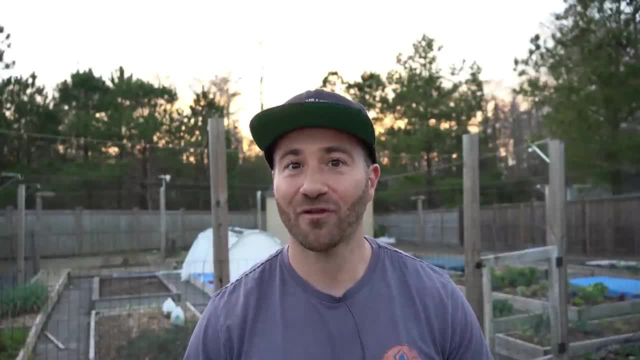 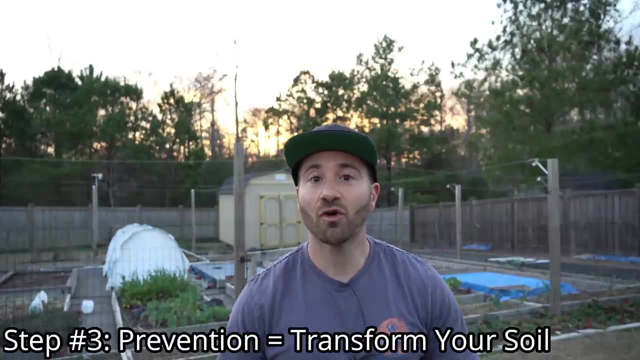 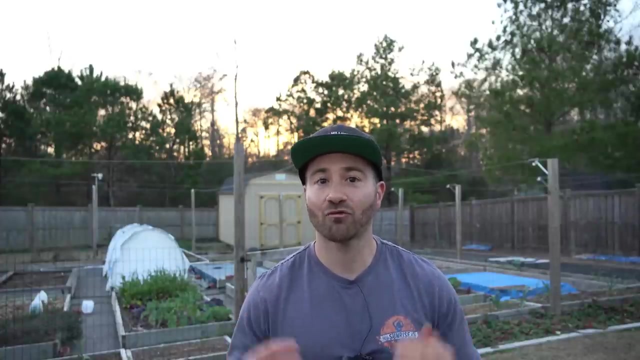 And I'm going to tell you exactly how to make your yard ant proof forever. The third step to make your yard ant proof forever is to change your cultural practices so the ants are no longer attracted to your yard, And that is to transform your sandy soil into an organic matter, rich loam. 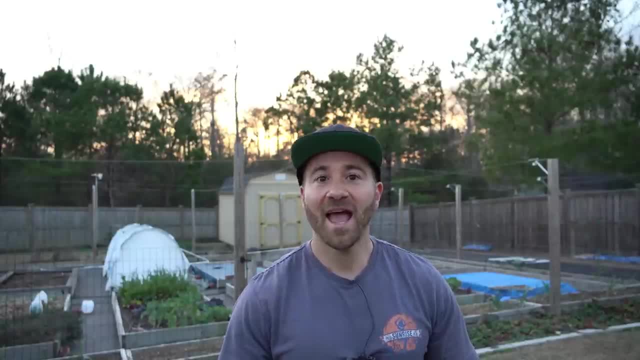 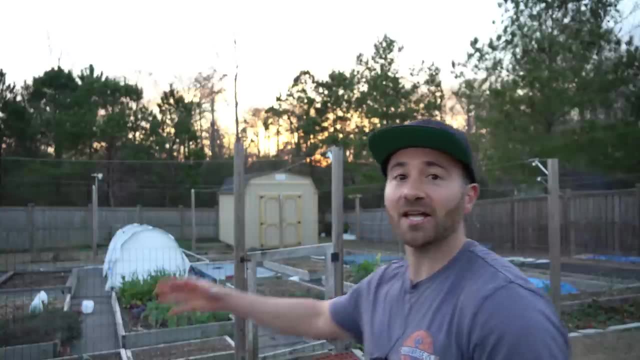 That is what I've done to my backyard. My front yard unfortunately has to stay a lawn due to HOA rules and for resale value of my house eventually in the future. My backyard, on the other hand, I've turned into a massive garden and an edible landscaping paradise, And I've added so much. 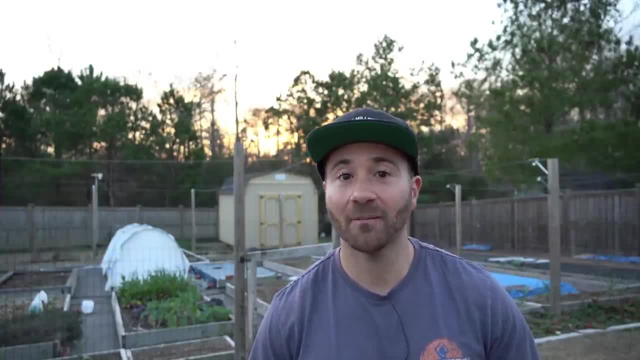 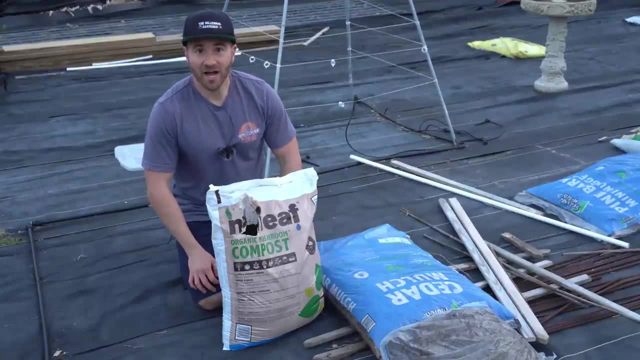 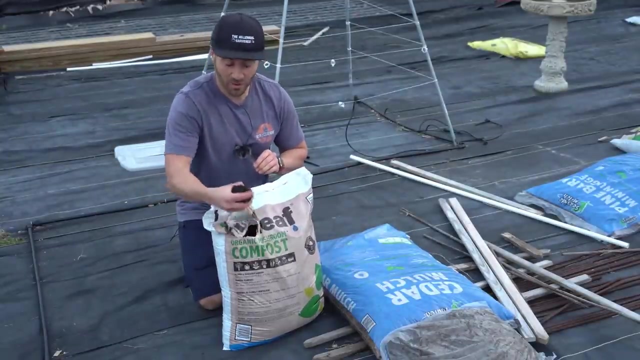 organic matter to my yard, that ants no longer want to come into the back, And I'm going to explain this in greater detail. As I mentioned earlier in this video, ants need to build their colonies in soil that drains well and holds structure, And they can't build in heavy organic matter, because 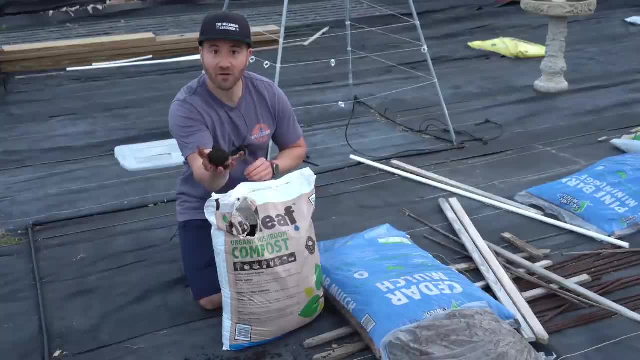 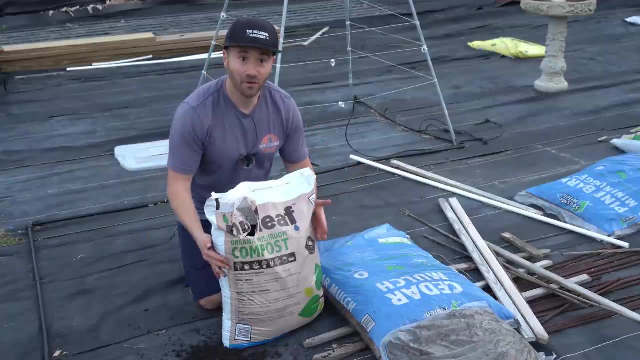 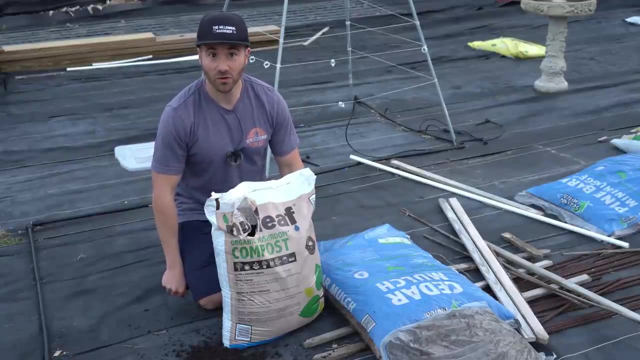 this stuff doesn't hold structure. It just completely falls apart. If they dig their tunnels in this, they're all going to collapse. So by simply adding lots of compost and mulch to an area, there will be nowhere that ants can build, And over time you will transform that soil. 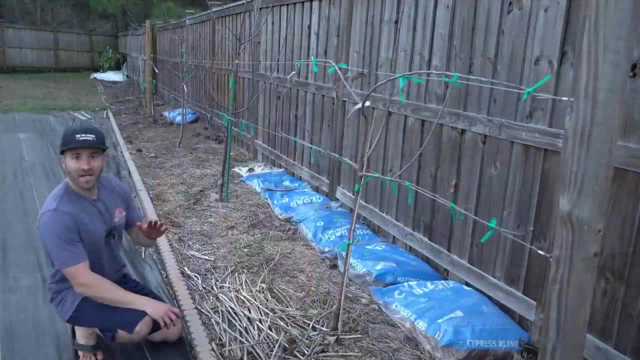 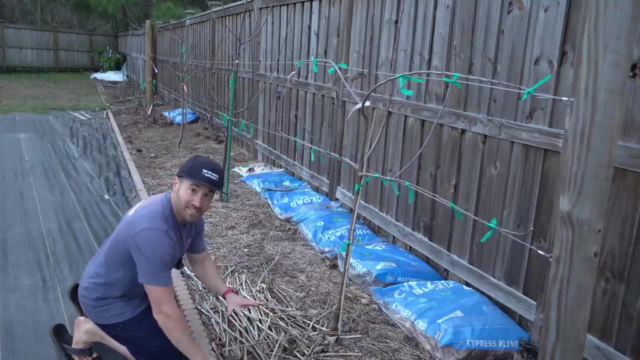 to a place that ants can never build a colony in, ever again. My entire backyard is lined with edible compost and mulch, And so I'm going to show you how I do my landscaping. I put these beds in everywhere, And on top of all of these beds is a four inch thick layer of compost and mulch. So if 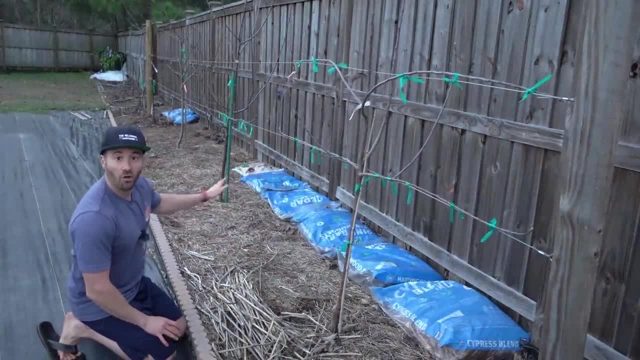 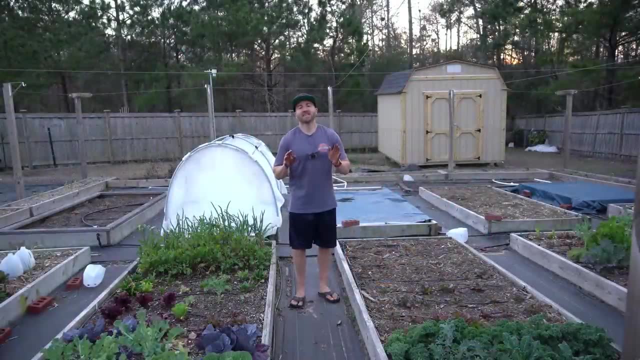 I dig into this soil, all I get is organic matter. There's nowhere for the ants to build all over the perimeter of my yard. It is off limits because it won't hold structure to form an ant colony. With my garden, I had to take a slightly different approach. All of my raised beds are filled with 100%. 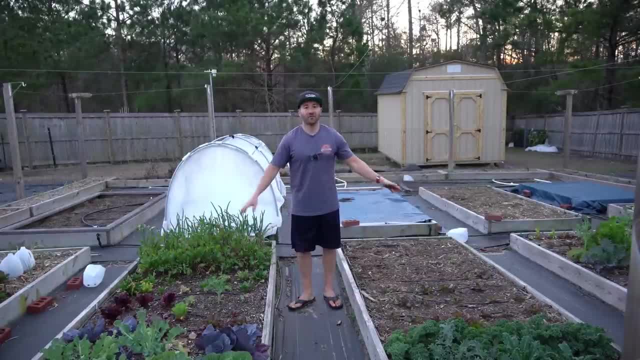 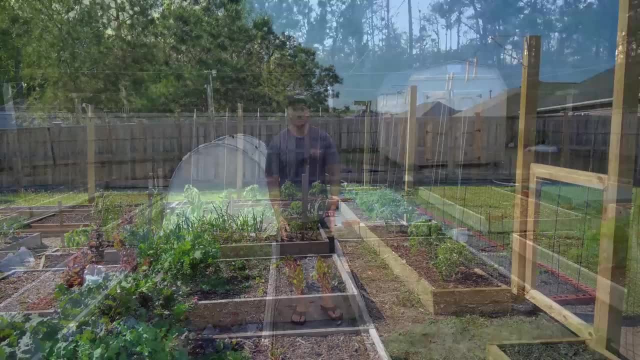 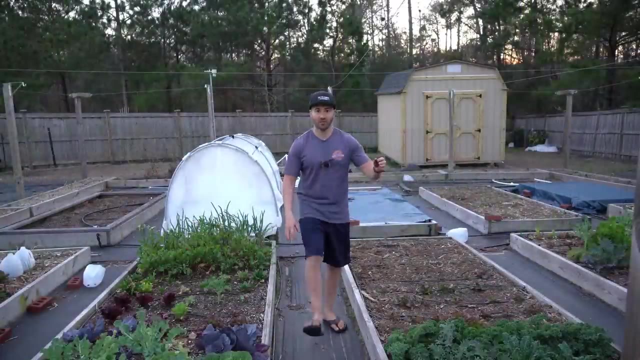 locally made turkey compost way ants could ever build in my garden beds themselves. However, it used to be that all of the walkways and rows in between the beds were the native sandy soil And as a result, they would be plagued with ant hills. And anytime I walked out into my garden with flip-flops on, I would get 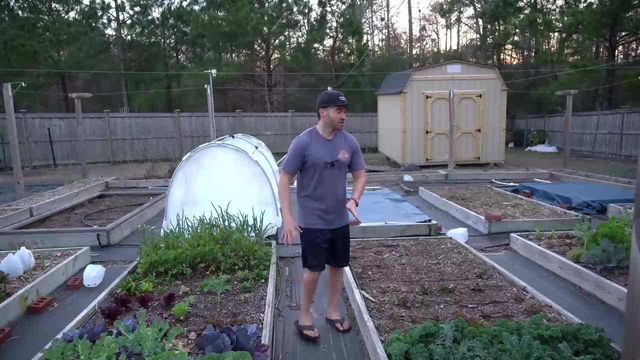 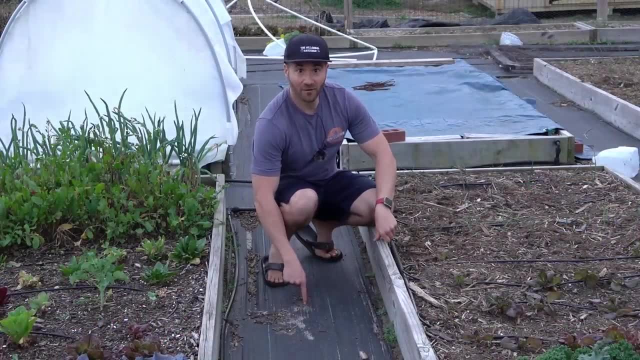 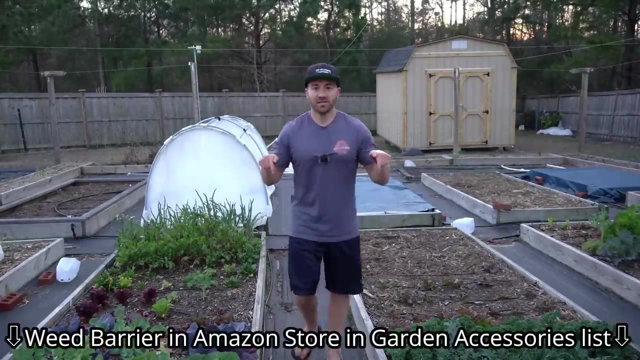 bitten by the various biting ants and fire ants that live here. So what I did was I lined this entire area with this weed mat, this weed barrier product, right here, And that has completely stopped the ants from coming and making colonies in my walkway, And I'll make sure to link to these. 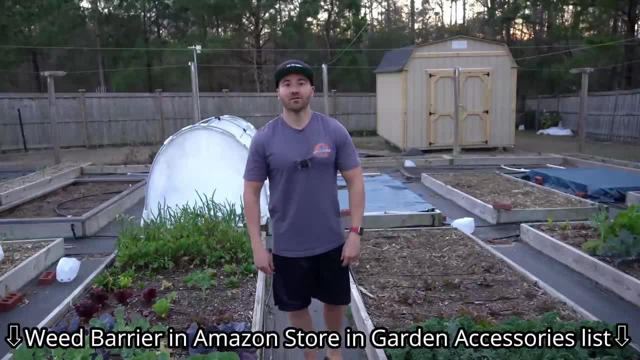 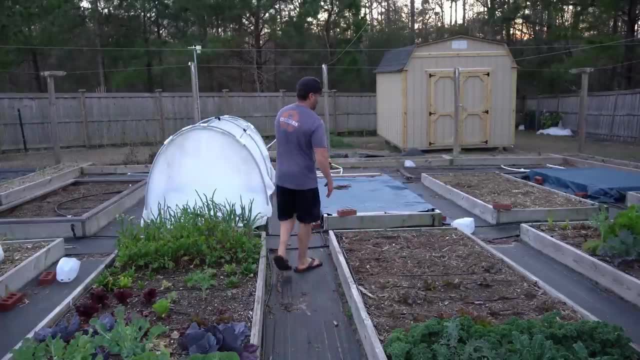 various weed barrier products in my Amazon storefront down in the video description underneath the category list garden accessories. So check that out if you want to buy weed mat, These weed mats, these weed barriers. they're all about five years old and they're still pretty much like new. 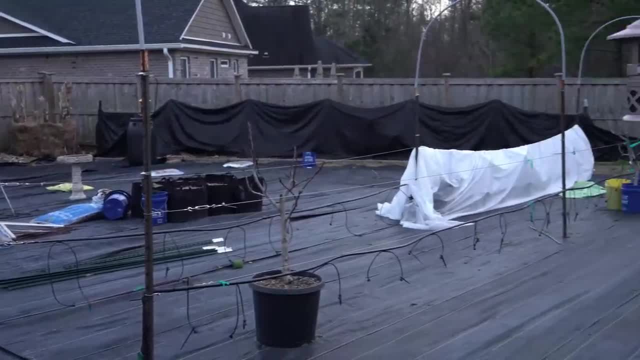 And I use them all around my yard. I really love them and I highly recommend them. If you have a problem with ants in your walkway, they are a great solution. So, between the perimeter beds, around the entire perimeter, I'm going to use a little bit of this weed mat And I'm going to use a little bit. 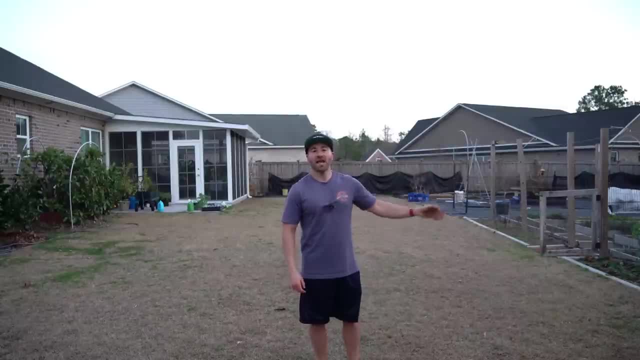 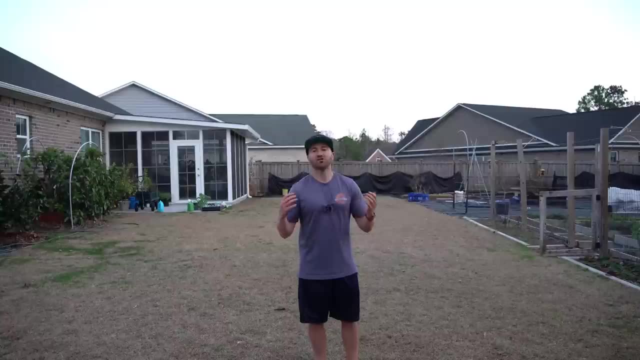 of this weed mat around the perimeter of my backyard that I use for edible landscaping and my garden area, and all the various weed mattings that I've put down. I've taken away all of the sandy soil that the ants want to build in, So there's no reason for them to come into the backyard, and 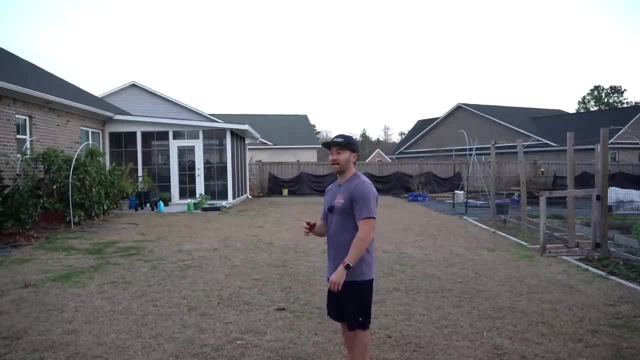 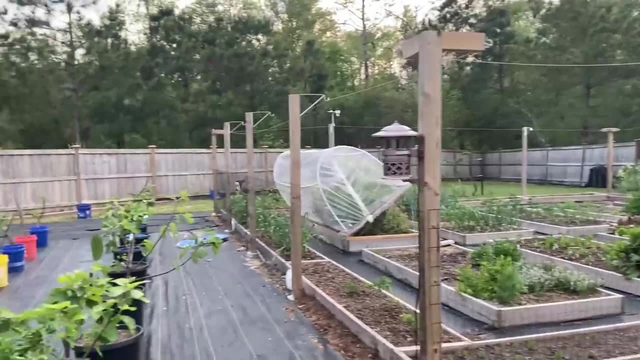 build ant colonies. The only place they can still build any colonies is this one strip of grass that I have remaining here, And the only reason why I maintain this is for my dog, Dale, so he can run around and do his zoomies. I just can't take this away from him, And I'm able to simply use those. 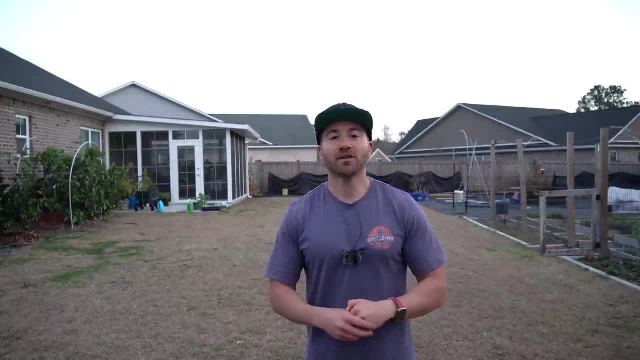 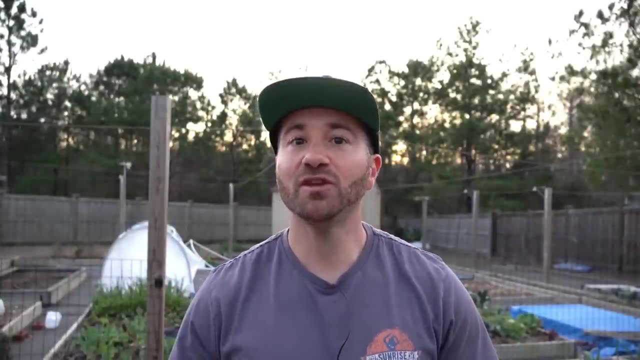 insect granules to control this area. by simply putting them down two to three times a year, This whole grassy patch right here remains ant free. So now that you've watched this whole video, hopefully you now understand exactly why your yard is so desirable for ants to build their 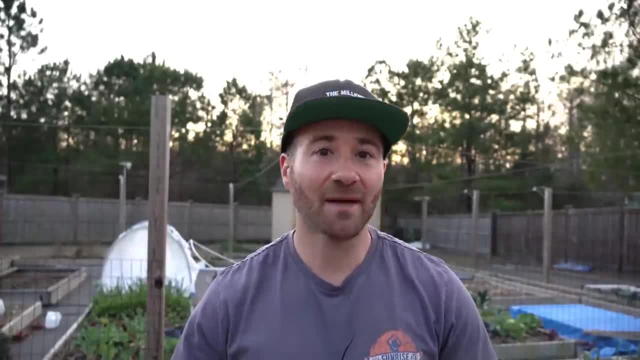 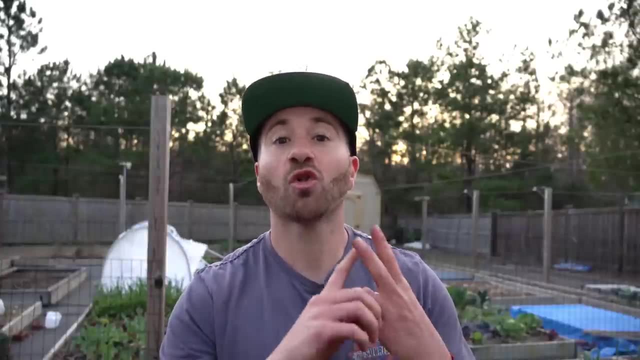 colonies in and take up permanent residency, And if you adopt this three-step process, that will help you deal with the ants both in the short term and transform your soil long-term, So you never have to deal with these ants desiring your property.